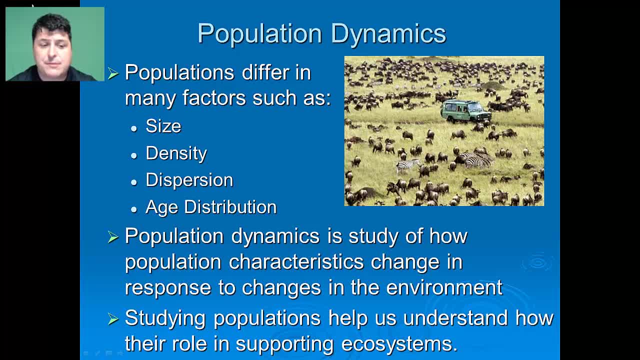 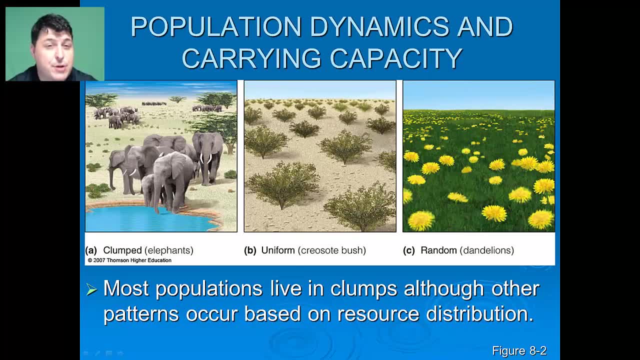 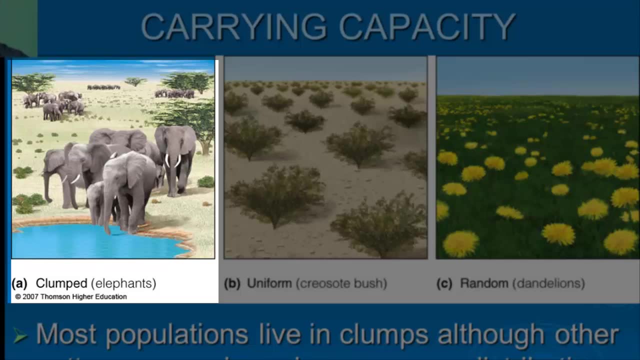 help us to understand their role in supporting ecosystems. Now, in terms of dispersion, depending upon where resources are, populations are going to be dispersed in various ways. Now most populations will live in clumps, Like the elephants in this particular illustration, But there are other dispersion patterns that 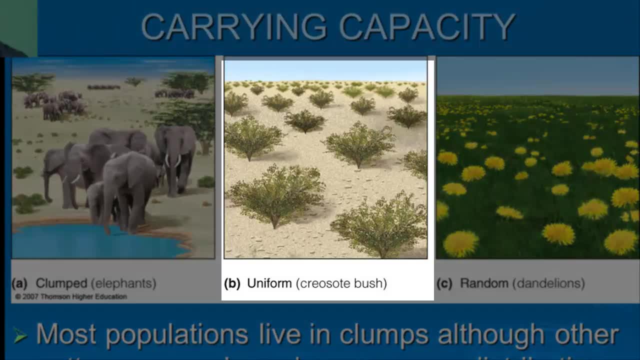 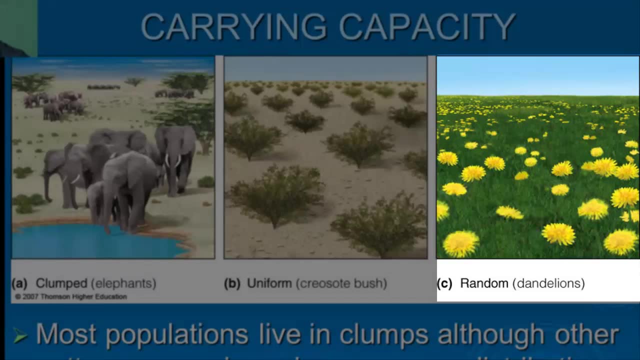 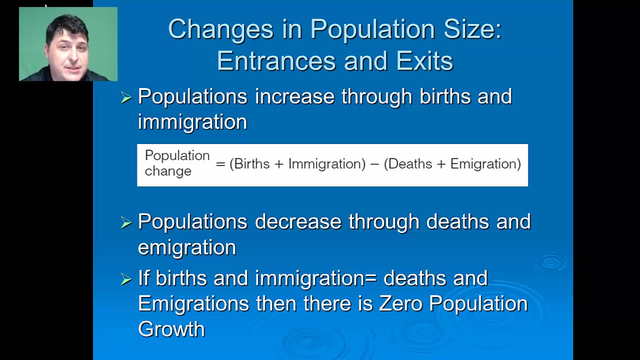 we might see from a uniform dispersion, like creosote bushes here, or through a random dispersion, like dandelions, And it's all based upon where the resources are for that population. Now, in general, populations will increase as a result of births and immigration. Those individuals 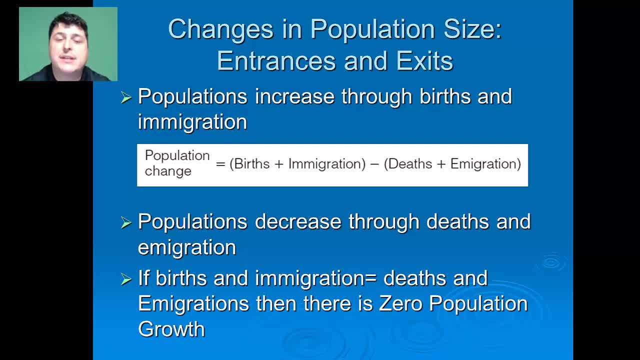 that are born and those individuals coming in are going to increase that population, Whereas populations will decrease when organisms die or leave an area through immigration. A simple formula can be generated in order for us to kind of recognize and see what would be happening to a population in a given moment. So the population change would be equal to 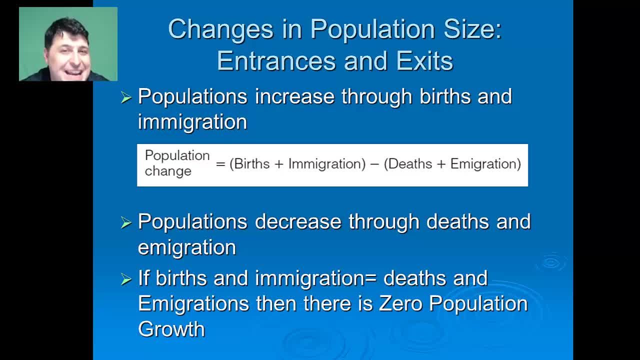 the births plus immigration, minus the deaths plus immigration. Now, if there's a situation where our births and immigration are actually going to be the same, then we're going to be in a very stable population where there's zero population growth, or ZPG, Now all populations. 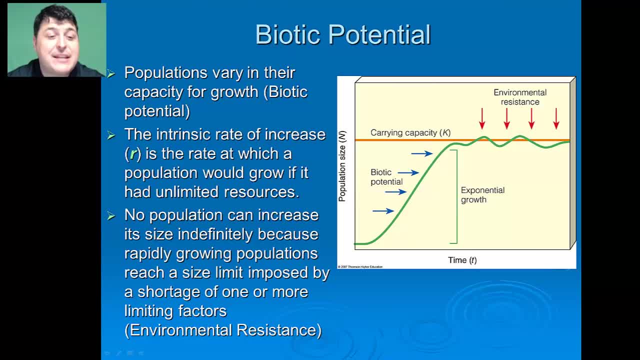 vary in their capacity for growth. This capacity for growth is referred to as its biotic potential. The intrinsic rate of increase would be the rate at which that population would grow if it had unlimited resources. How fast that population would increase over time would depend on the size of that population. Now, typically, no population can increase indefinitely. 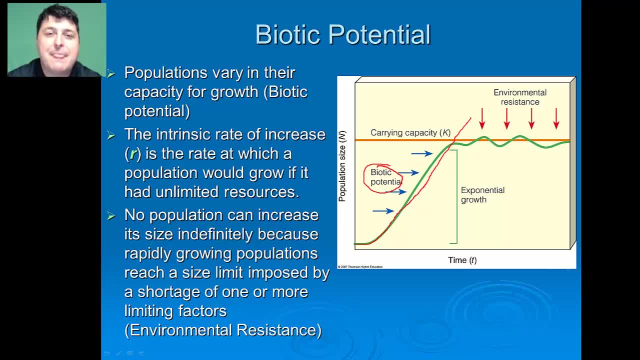 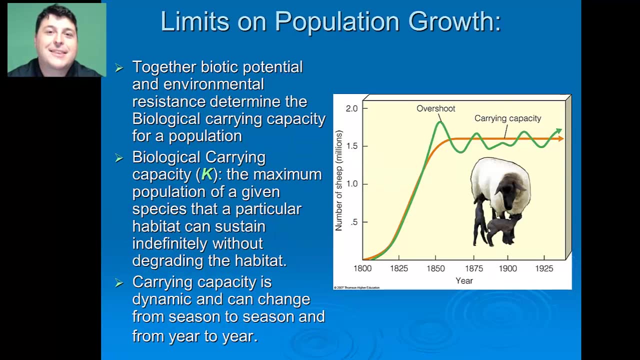 because rapidly growing populations will reach a size limit that's imposed by a shortage of resources or one or more various limiting factors. These limiting factors are referred to as the environmental resistance. So together, the biotic potential and the environmental resistance are the two main factors that are going to be used to establish. 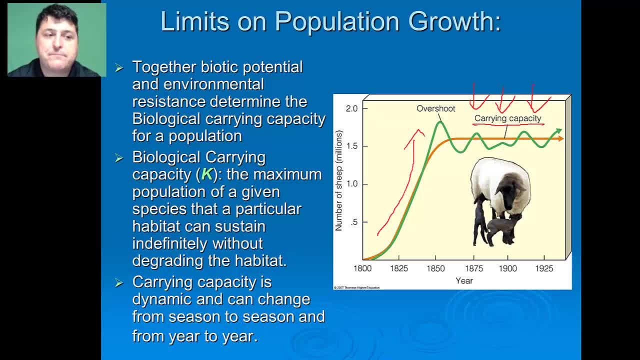 the caring capacity for a population. The biological caring capacity for a population would be the maximum population of a species that a habitat can sustain indefinitely without degrading that habitat. So you might reach a point where you have a maximum number that there could be in an area. but if that maximum number can't be sustained, well then you're. 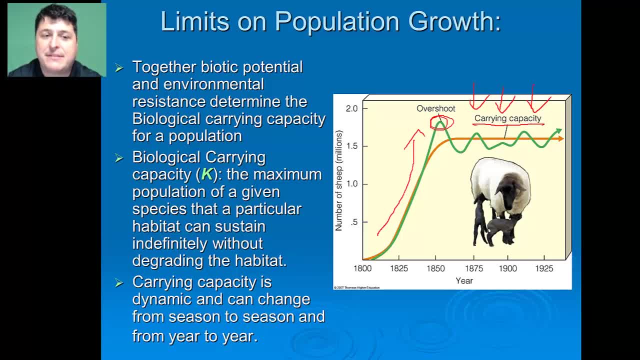 going to have a large amount of habitat that's not carrying capacity. Now most populations will hover at or around that caring capacity and will have kind of that theoretical caring capacity, which would be that average number of individuals that we're going to be able to establish in that particular area. One important thing is that caring capacity is. 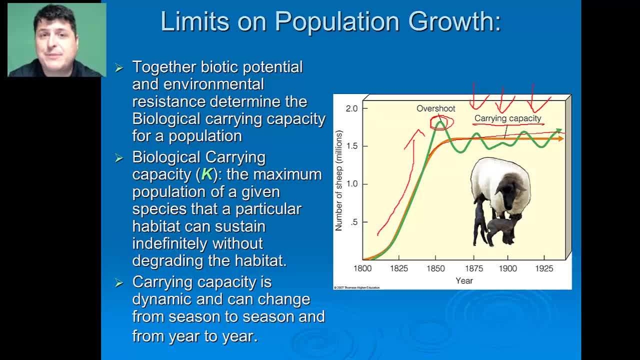 not static, It's actually dynamic and it can change from season to season And like, for example, with sheep, if we have a really rich spring with lots of rainfall, so we have lots of grass, we might have a high caring capacity. But the next year, as a result of 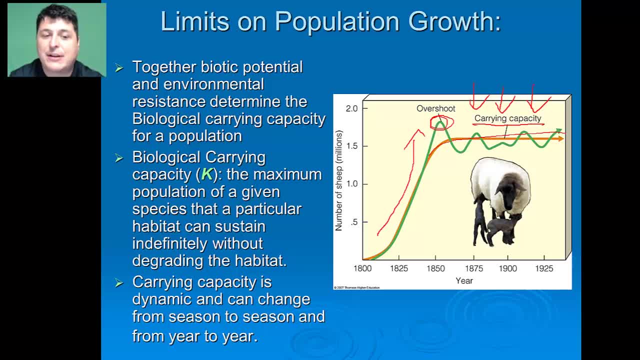 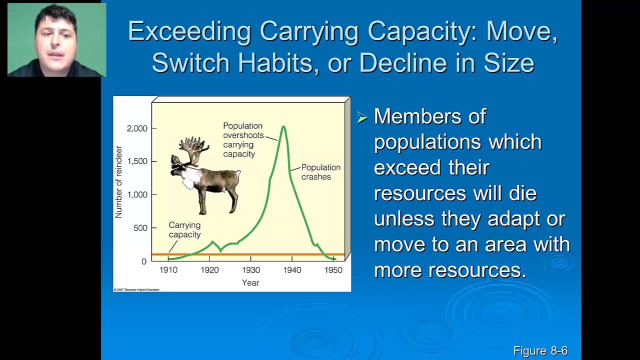 drought, that area might have a much less caring capacity and so the caring capacity for that environment might shift depending upon the environmental conditions and the environmental resistance which is then present in that area for that time. Now, any population that actually exceeds that caring capacity is going to die, and they're going to have 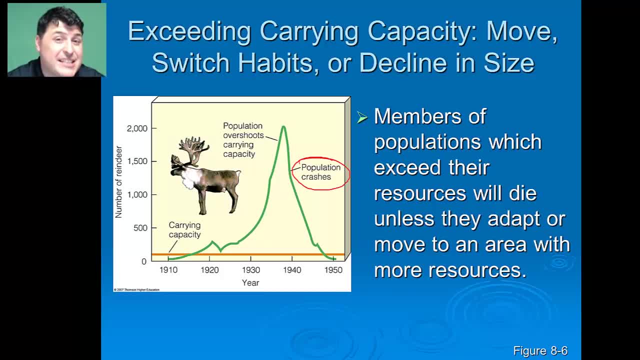 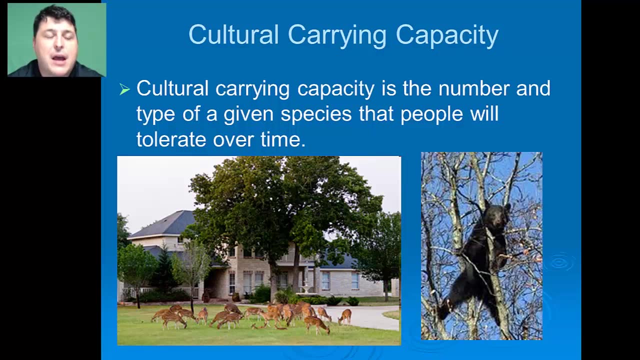 basically a population crash unless they're able to adapt to those changes or move to an area with more resources. Now there's another kind of caring capacity that we want to speak of here, but it'll become more important later, and that's the idea of cultural caring capacity. The cultural 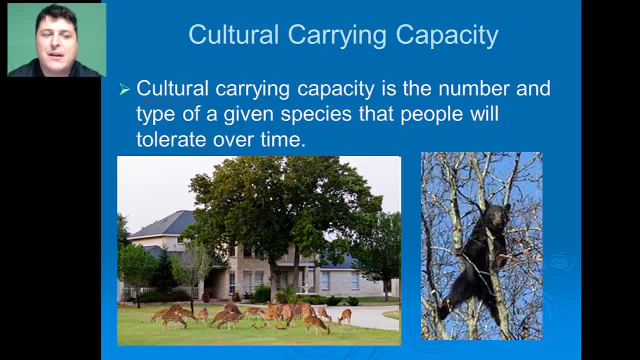 caring capacity is actually the number of a particular species that the people can tolerate over time. So, for example, an area can support a whole bunch of healthy deer in the environment, but as a result of the people not wanting the deer around because of car accidents, 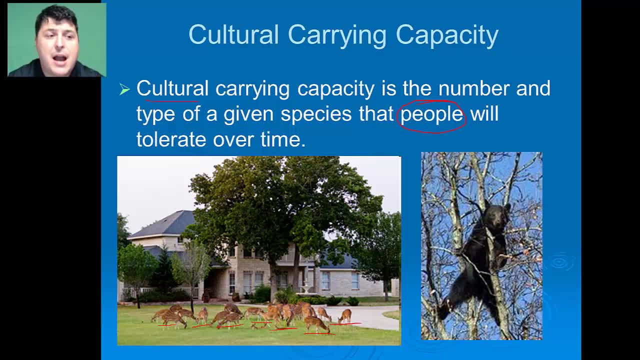 or them eating their expensive shrubbery. the cultural caring capacity might be much less than that of the biological. So what can we do? We can do a lot of things. The biological carrying capacity, Now some of the limiting factors that are part of 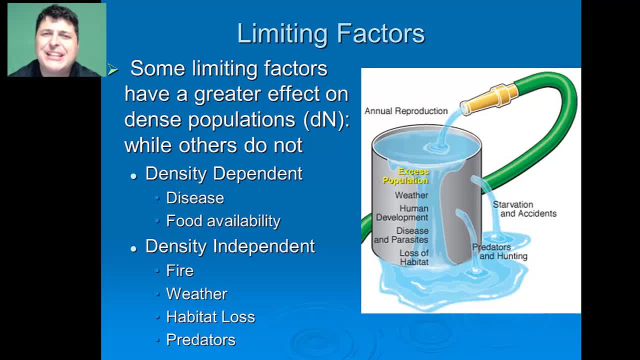 that environmental resistance have a greater effect on really dense populations when you have a lot of individuals in close quarters in a small area. Some density dependent factors that are going to influence and impact more dense population more so than a less dense population will be things like: 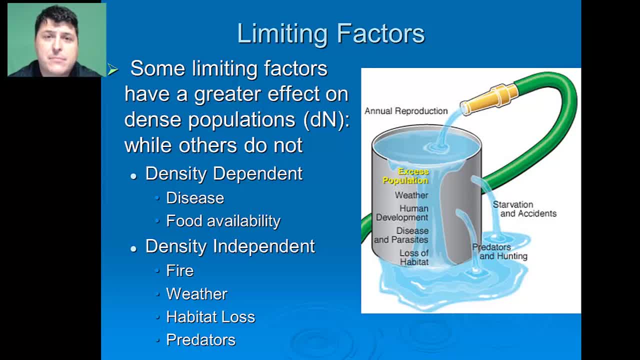 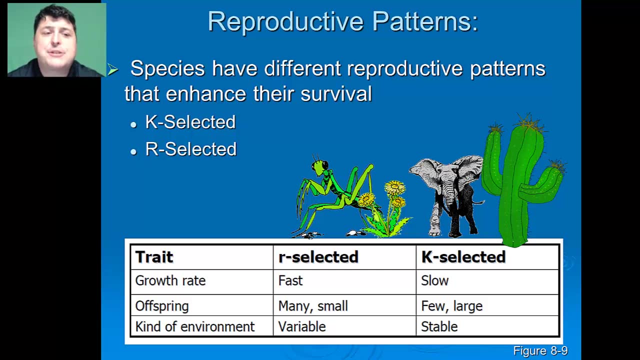 disease or food availability, whereas things like fire and weather and predators will equally impact individuals that are dense or less densely populated. Now, a lot of species actually have different reproductive patterns that will enhance their survival. the two major reproductive patterns that we'll want to look at are case selected and are selected species. 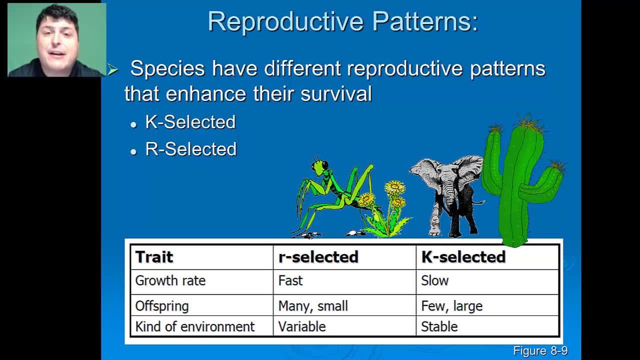 Our, Our selected species have a very fast intrinsic rate of increase. They have a very fast growth rate. They're going to have lots of babies, lots of offspring, but they're typically small and they're able to live in various environments, even environments that are highly changeable. 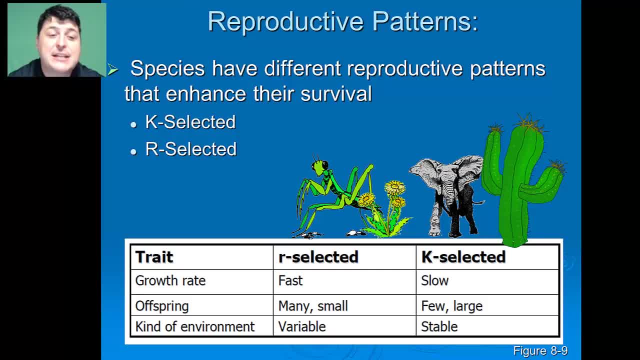 Some great examples of our selected species would be like insects or dandelions. K-selected species really have a slow growth rate, so their intrinsic rate of growth is going to be very, very slow. They typically have very few offspring and the offspring are large and they require. 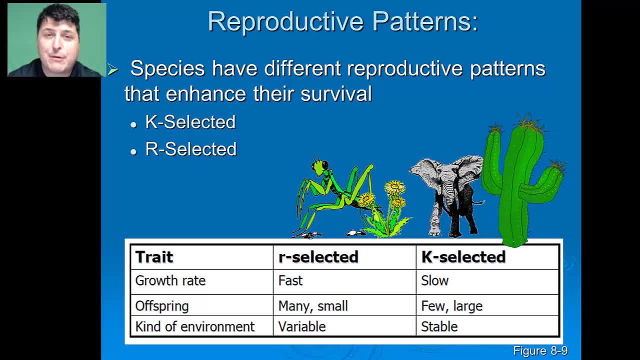 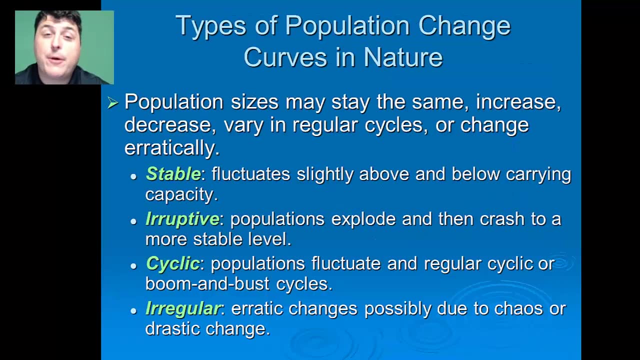 additional kind of parental care, either before birth or after birth. And then they need to exist in stable environments because their populations stay at or around the carrying capacity, and that's why they're called K-selected species. Depending upon the environment, population sizes may change. 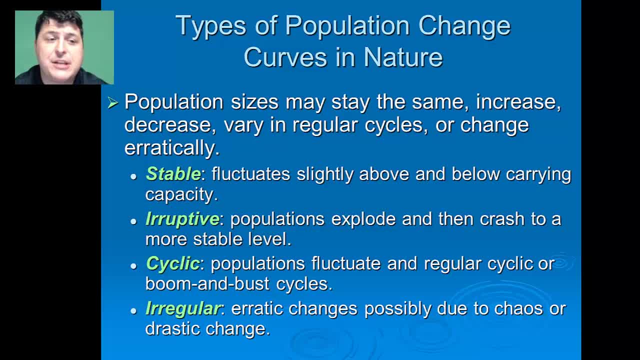 They could stay the same. They could have great increases or decreases. They could be more cyclical or have very erratic changes. Stable populations are those that fluctuate slightly above and below their carrying capacity. We see a lot of stable populations in more stable environments, like that of tropical rainforests.